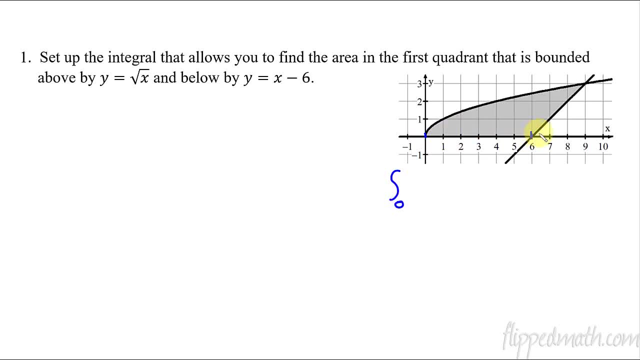 I'm going to repeat that. I start it here, at x is 0, and then I go up to where x is 6, and then it's this graph on top which was the square root of x, and then you subtract the graph on bottom, which in this case was nothing. So then that's that with respect to x, And then you add the second integral, which was starting at 6, and you go until you get to 9.. And then again it's the square root curve on top, and then you subtract the thing on bottom which was x minus 6.. 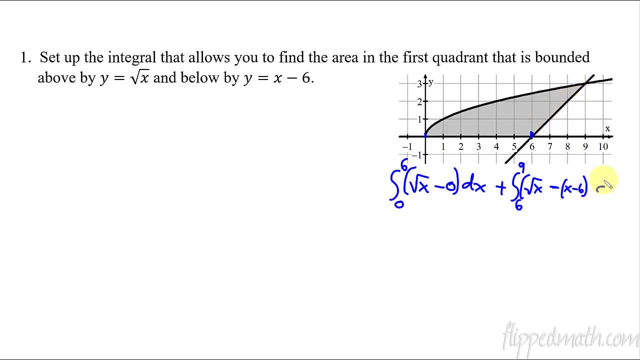 That's the square root of x, That's the boundary, that's on bottom of this area, And that's all again with respect to x. All right, so that's what we did before We started, with our small x, go to our large x, depending on how the region is divided up. So now let's figure out how do we do this. with respect to y, The first thing you have to do is take these equations and change them so that they are, in terms of y, meaning solve for x. If I square both sides, you'd end up with y squared equals x. So there, now we have x equals. So this graph right here. 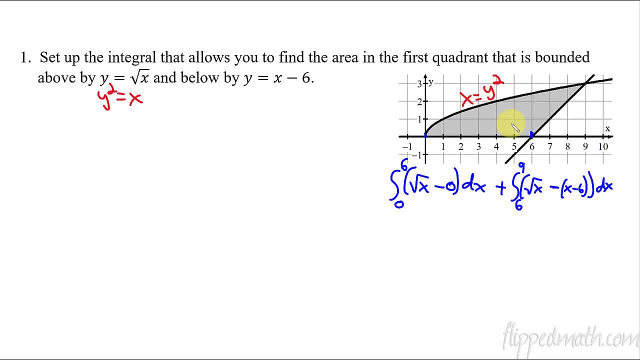 Represents y squared. It's x equals y squared. That's this graph, this graph: here, if you solve for x, I would add 6 to both sides, you to end up with y plus 6, and there that is this line. So I could say: this graph represents x equals y plus 6. 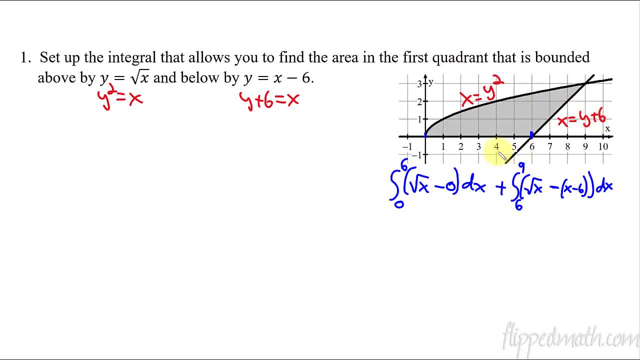 So we're so used to thinking of graphs in terms of x, where it's always y equals. But it doesn't have to be that way. these graphs could also- we could flip it around and make it be x equals. So this x equals y squared. this piece of this graph is exactly the same thing as y equals the squared of x. 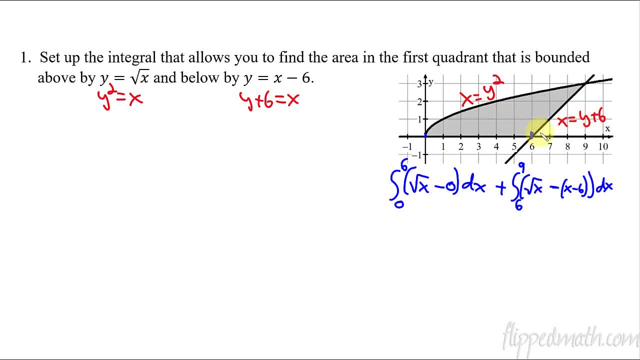 Same with this line: here, x equals y plus 6. Okay, now we have it in terms of y, so we can set up an integral in terms of y. This is cool, I love this. So you take the integral And you look at this thing. you think what is the boundary on the right side of this area? 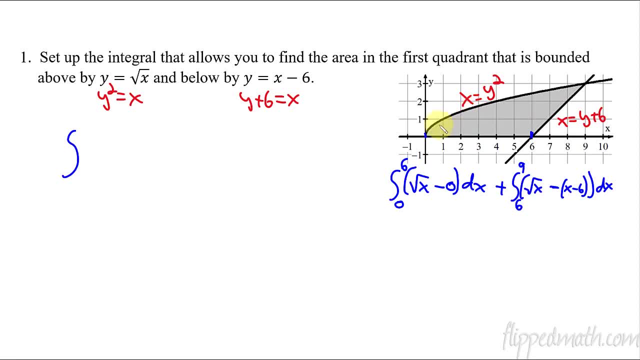 That's what you start with. see, before, when we did the x, we started with the graph that was on top, the one that was above. but No, you're doing with respect to y. you think which graph is the one on the right side. So the boundary of this is that on the right side is just this one line, and so it's y plus 6. 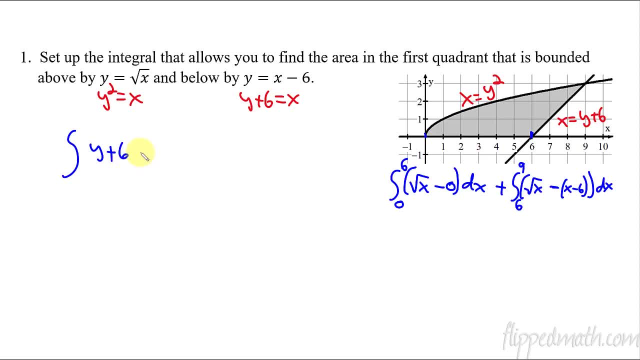 That's what we start with: y plus 6, and then you subtract the graph that's on the left. So here's the graph on the left, this y squared graph. So we subtract y squared. Now what about the boundaries? before we did 0 to 6, we did x value from 0, x value to 6. 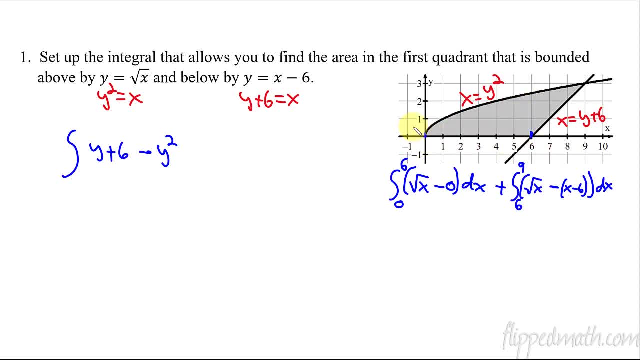 Now for this region. We're going to do this. We're going to do the y values. the smallest y value of this region is a 0 and the highest y value of this region, Which is right there, that y value, is a 3. So this is the setup, and then you say with respect to y instead of with respect to x, and then that's it. 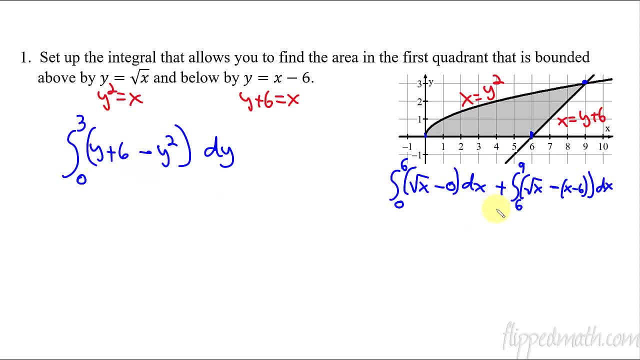 This integral and this integral are exactly the same thing. They equal each other. if you work this out by hand, you'd see that this it's the same thing as this one. Now, this is kind of nice because with this example with respect to y, is a much simpler integral to work with. 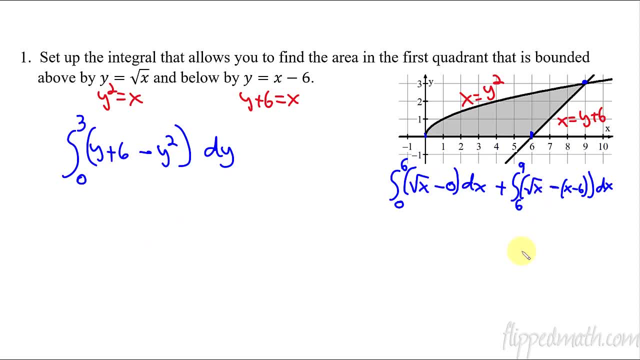 As opposed to this crazy stuff over here, And that's why, at sometimes, we'd rather work with respect to y in certain situations. Now let me just say though, real quick, before we go on to some other examples: if you were to use a calculator, You know your math 8 stuff or, excuse me, math 9, math 9 in the TI 84 where you set up the integral. 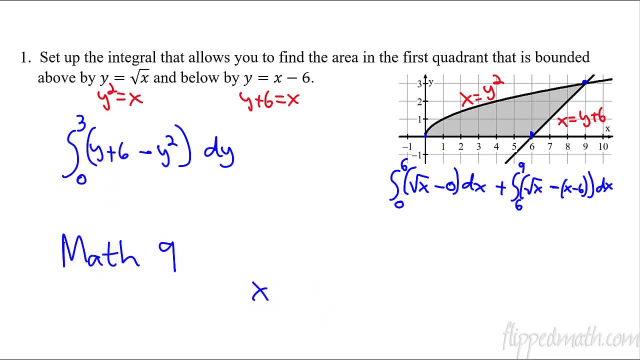 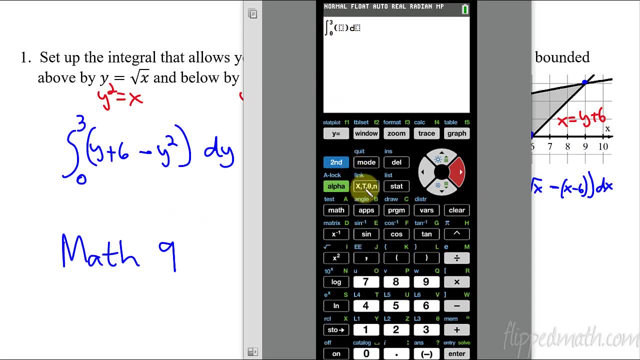 When you push the XT theta button here, let me just pull it up and show you there we go. So we got some 0 to 3 and then we'd say here we would not have, we would not say why, we would just push This button right here, the XT theta n button. 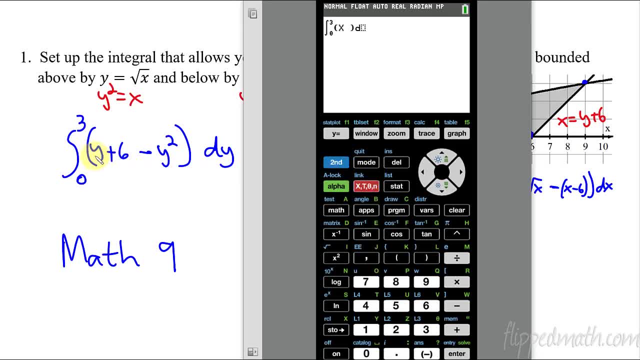 This is a variable, button it. the calculator doesn't care if it's a Y variable or not, You just use variable. so just don't get that confused. and then so you'd say: X plus 6 minus x squared. And then here of course you'd have to say, with respect to X, 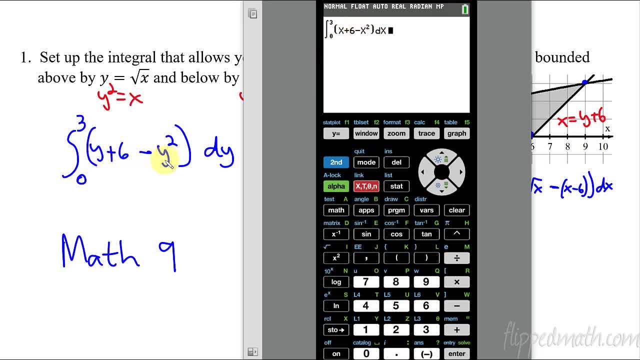 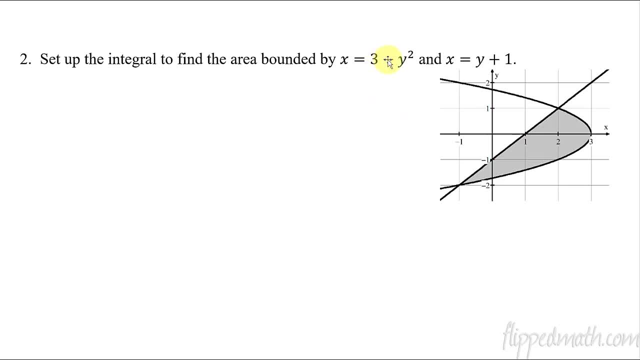 So if, when you're using the calculator, you still use X's, even though here it says Y's, because this X just represents It's a variable. Okay, Let's move on to our next example. This one's a little easier because I gave it to you in terms of Y, So it's X equals, this one's X equals. 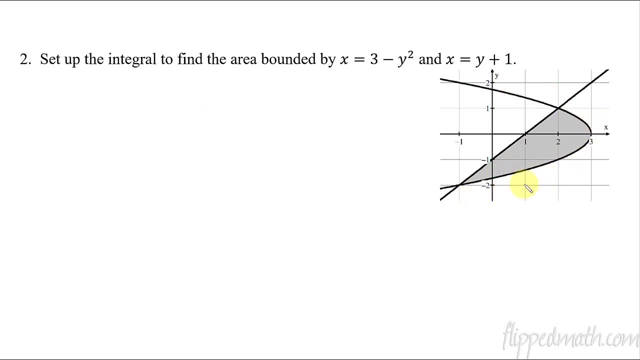 Let's just make sure we know which one is which. so this little parabola looking thing, The sideways parabola, is X equals 3 minus Y squared, and then this line is the Y plus 1, but I'm gonna leave off the exit. Well, now put it there: X equals Y plus 1.. That's the straight line here. 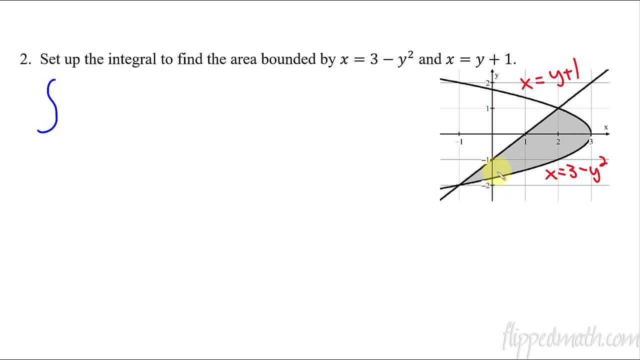 So let's set up our integral now. Do we need one or two integrals? Let's look at the right side. This is the curve on the right side and it never changes. It is 3 minus Y squared everywhere on the right side of the shaded region. now. 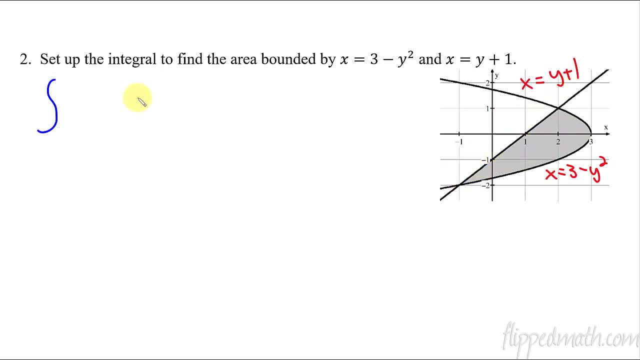 Let's look on the left. The left side is this flat line the whole time. So we only need one integral to set this up. The smallest Y value is right there, That is a negative 2. The highest Y value is right there, and that is a 1. and then we do the graph. 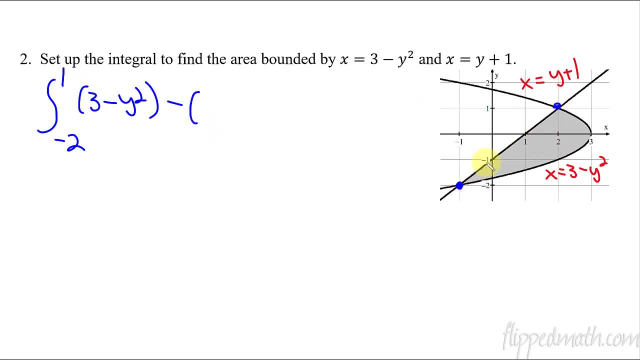 That's on the right and subtract the graph That's on the left. That's it would be the smaller region, and then that is with respect to Y, and you could simplify this. Let me just simplify that real quick. I put the Y squared in front. So there that. 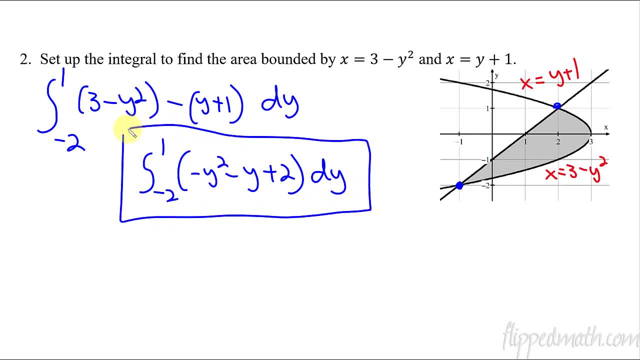 Is what it simplifies to, so that integral represents this area. So once you get used to this, it's pretty fast and easy. You just have to think a little bit differently, because you're thinking the right side of the region and the left side of the region. 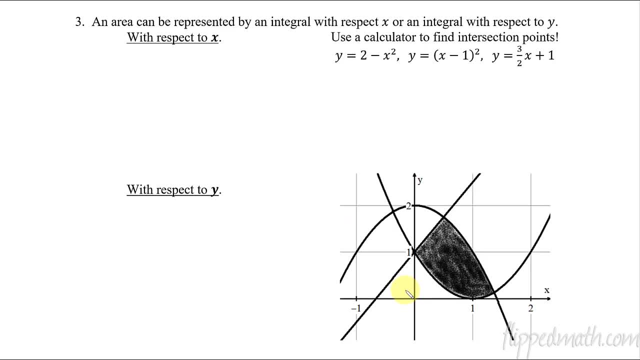 Okay, let's do one more. That's a bit more challenging, And this time we're going to set up the integrals with respect to X and the integrals were with respect to Y. In order for us to do that, we need to know all of these different. 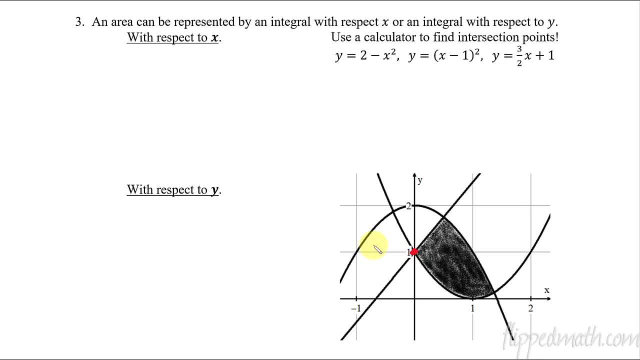 Intersection points of this strange thing. So this one's easy, that one right, there is just 0: 1, and then that one: there is 1: 0, but we need the this one and this one, Okay, so I'm gonna save you some time. 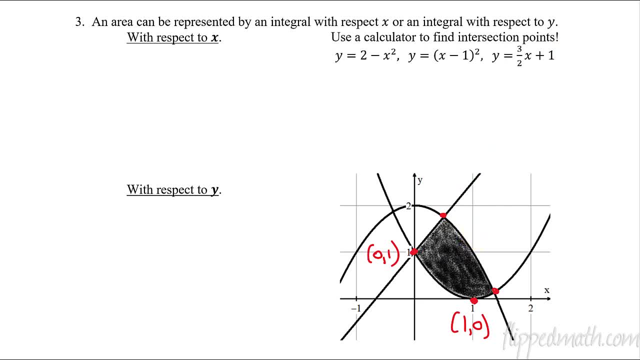 I've already done it on the calculator. I'd graphed them and figured out the point of intersection. So just write these down. this one on top is 0 point 5 comma, 1 point 7, 5. That's where this intersection is, and then this intersection point right there is 1 point 3, 6, 6, 0, 2. 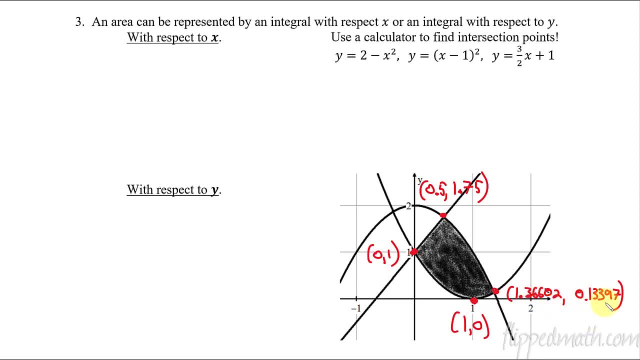 I tried to write several decimals and then the Y value is at 0 point 1, 3, 3, 9, 7, All right, so you get those written down and now let's start setting this thing up. So we start with respect to X. We need to think. 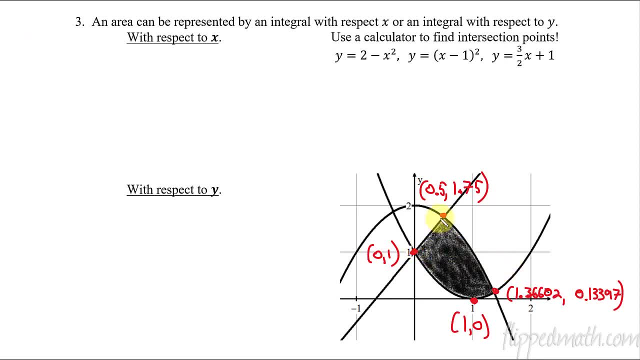 We're going from the left to the right, But as you move from the left to the right, the the graph on bottom is the same the whole time, But the graph on top changes right here. So I'm gonna draw a little line right here to remind myself that I'm doing two separate integrals. 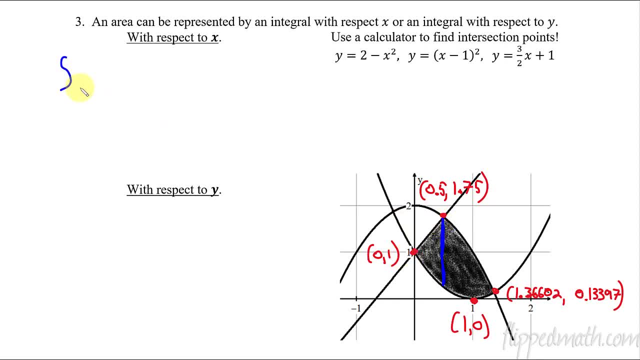 So I'm going to do an integral from 0 to 0, point 5, and I take the graph That's on top, which is that line Which is 3 halves X plus 1, and then you subtract the graph that's on bottom and this parabola here is: which one is that parabola? 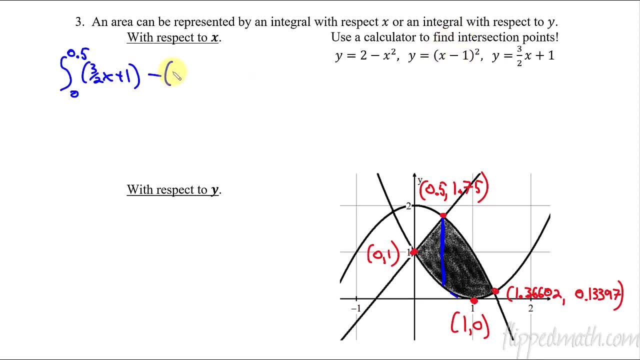 that's This one right X minus 1 quantity squared, and then that's all with respect to X. So that's just my first integral. That's just this piece that I just did right now. Now I'm going to add the Integral of the second piece here. 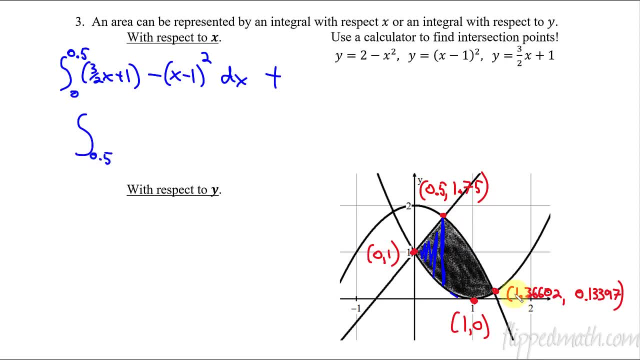 So again, I'm starting at 0 point 5 for my X value and I go up until I get to this weird decimal, 1 point 3, 6, 6, 0, 2, and the graph on top is this parabola. that parabola is which one? 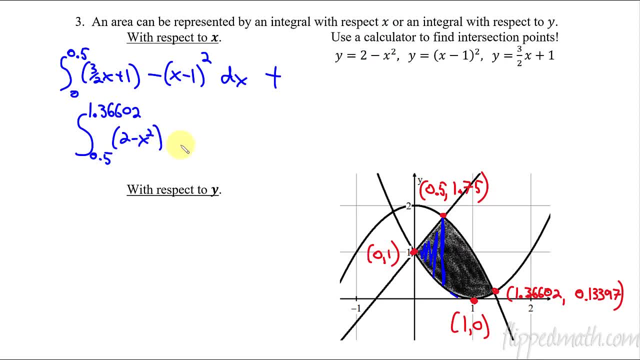 it's this one: 2 minus x squared. so I start with 2 minus X squared And then I subtract the one that's on bottom, which is that parabola quantity x minus one squared, And then that's again with respect to x. So there's my two integrals. that would 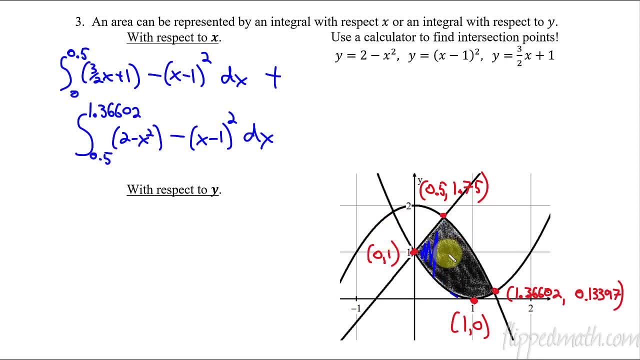 represent these two regions right here. Now let's set this up with respect to y. So I'm going to erase my blue stuff here and restart this with respect to y, And as you do this, now we have to think differently. You're thinking: what is the right side of the graph? The right side is this: 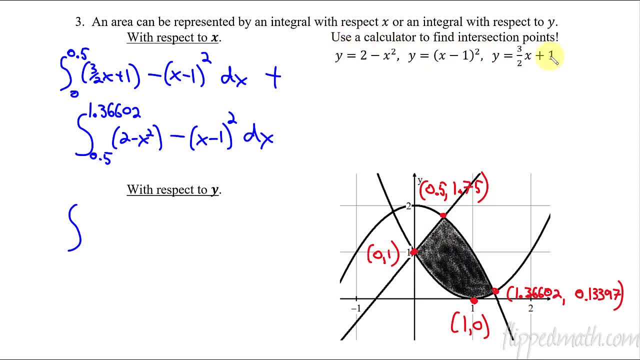 curve here. Oh, we can't even do this yet. Hold on. We got to change these equations so that they're in terms of y, So solve for x. I'm going to add the x squared to the left side. subtract the y. 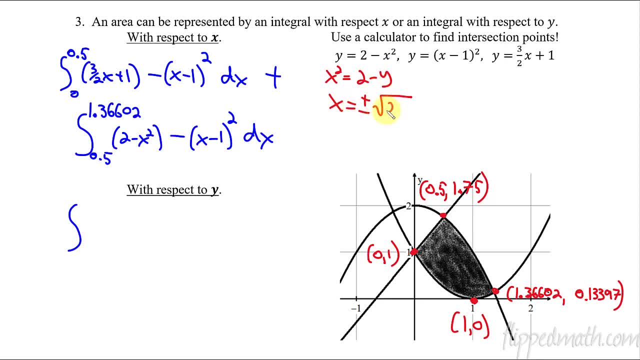 and then I get: x equals the square root, gives me plus or minus the square root of two minus y. Now, the reason it's plus or minus is because this parabola right here, the one that we're working with, the left side of it is the negative square root, The right side of it is the positive. 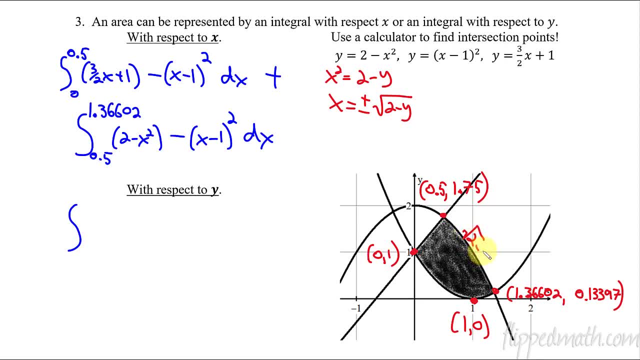 square root. So this right here is the square root of two Minus y, all underneath the radical, but it's the positive side. This side over here is the negative, So we don't even need that one. So we only need the positive square root of two minus y. 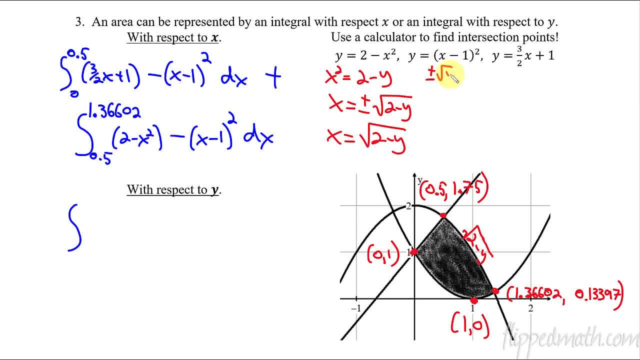 Okay, next one: Here you take the square root of both sides. So again we're going to get plus or minus the square root of y equals x, minus one. add the one to both sides, So this is going to give me x equals plus or minus the square root of y, plus a one on the outside of the radical. So why is it? 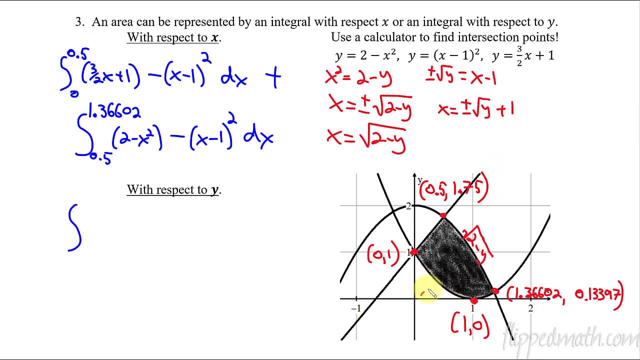 plus or minus. Again, the left side of this would be. so this right there would be negative square root of y plus one, And this side, right there would be the positive square root of y plus one. What's left? I need this one. I got to figure out what that is. I'm. 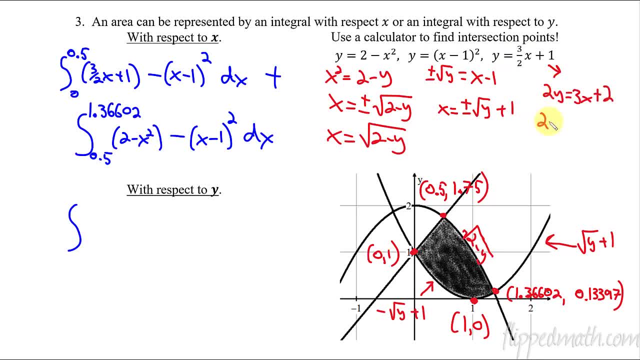 going to multiply by two to get rid of the fraction, And then I solve for x. So there's my x, And what is this? That's this line, right there, That's that flat line. So this part, that's what. that's what's going to come in handy when we get to there. Okay, now, this one is as hard as you're. 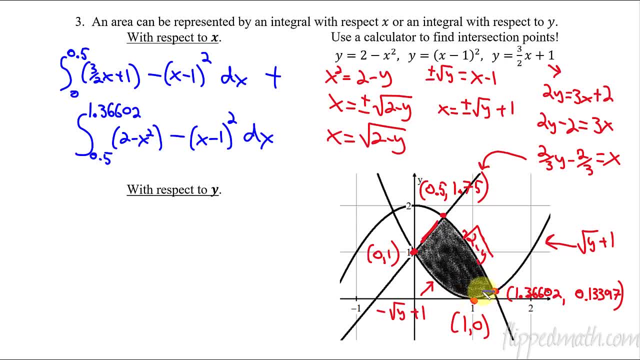 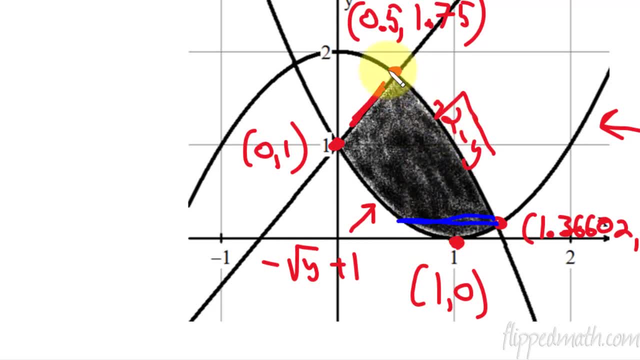 not going to have one on a test that's nearly as hard as this one. I just wanted to show you a pretty challenging one. This is tricky because there are three different regions. You see here this on the right side and on the left side. when you start comparing, right side of the area. 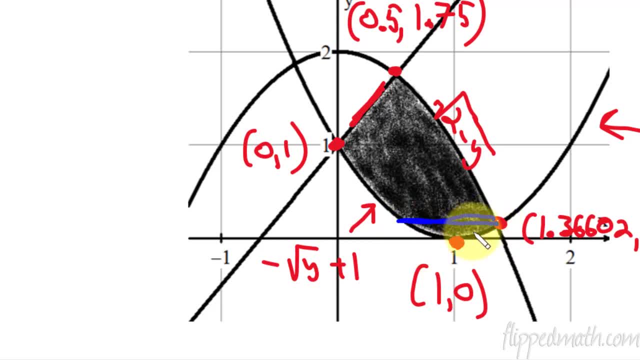 the left side of the area. this right side changes right there. It is this graph first, and then it changes to this graph And then it changes again here. And why does it change there? Because the left side of the graph it's this parabola at first, and then it changes to this line. So we 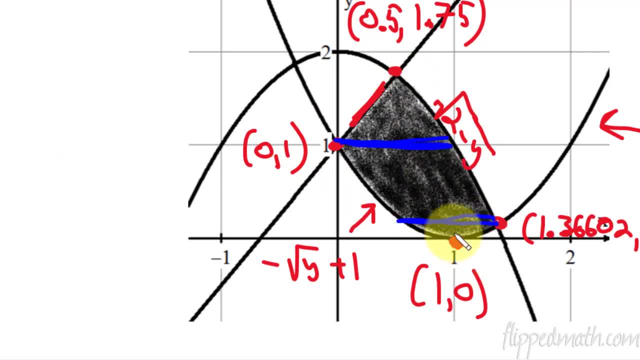 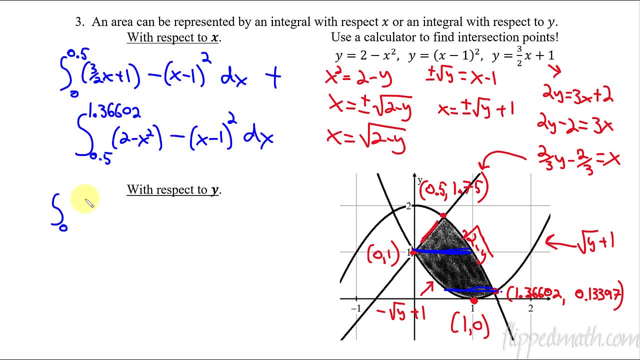 have to do three integrals, And then we have to do three integrals, And then we have to do three integrals. Holy cow, All right, let's set this up. So our first integral- this region is the bottom of it- is a zero. And then what's the top of it? It's this y value right there, 0.13397.. And 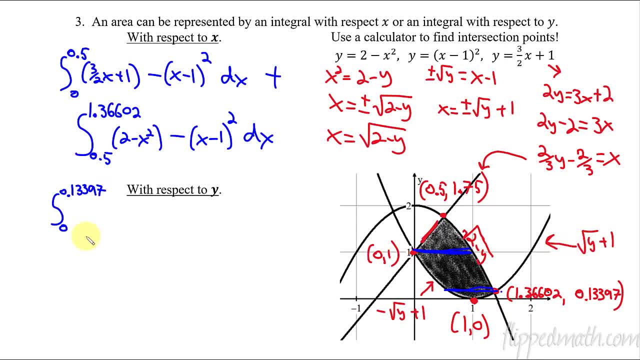 then we take the right side, which is this positive square root of y plus one, and subtract the left side. this part right here is the negative square root of y minus plus one with respect to y. And yes, we could clean this up. We're not going to worry about this for the lesson. We're just trying. 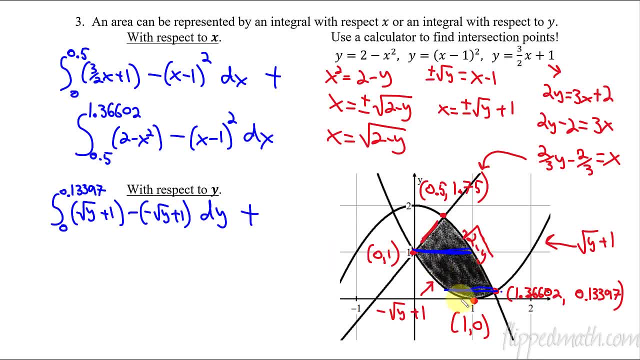 to figure out how to set up integrals, And then we're going to do three integrals, And then we're going to do three integrals, And then we're going to do three integrals And then we say, plus, now let's do the next. So we just did this one, That's the one we just did. Now let's do this region. So 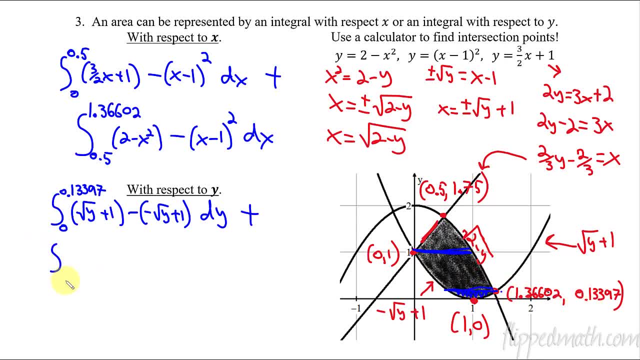 we go, the smallest y value here again is 0.13397.. And then it goes up until we get to a y value of one. And then you start off with the graph that's on the right side, which is the square root of. 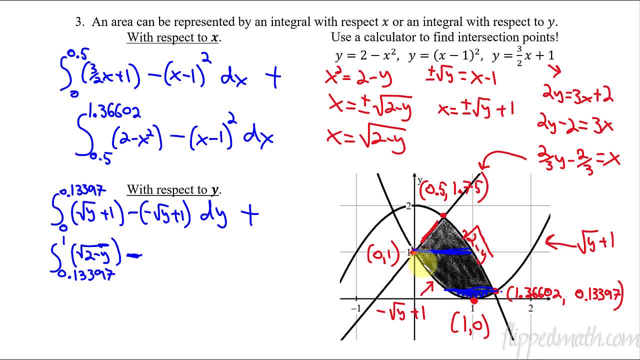 two minus y. And then we subtract the graph that's on the left side, which is this thing again negative, square root of y, plus one on the outside with respect to y, And then plus again, holy cow. And then we have one more region, which is this top region. 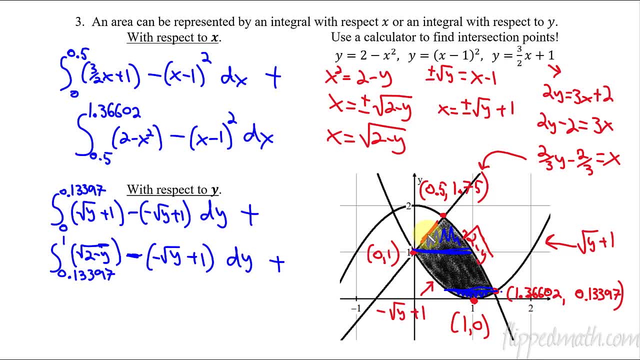 And why is it another one? Because we are changing the graph. the boundary on the left side, that left boundary, is no longer this parabola, So the right side is still this thing. Oh, we got to set up our integral first. So the bottom of the integral is a y value of one. 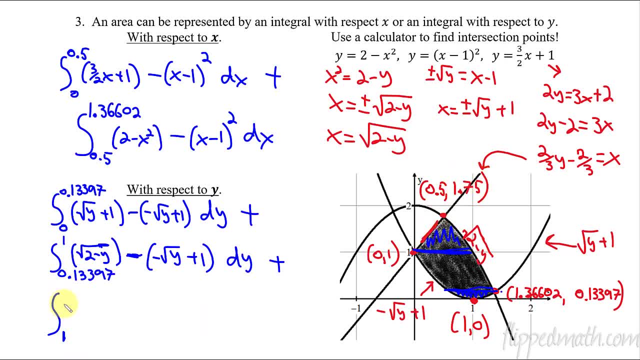 And the top of the integral, the top of the boundary, would be a y value of 1.75.. And then we start with this part of the parabola here. So we're going to say square root of two minus y And 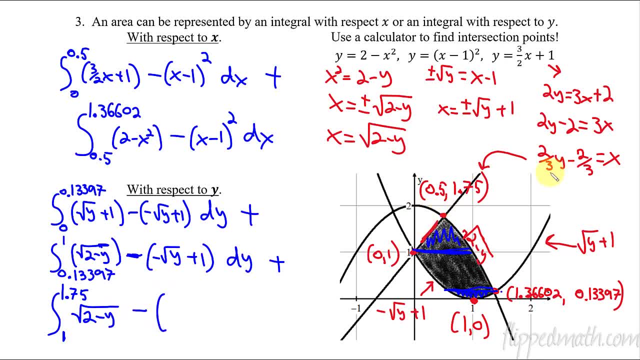 we subtract in parentheses the line and the lines equation is this: right there, with respect to y Holy cow, That is a mess of a problem. Okay, This is. you're never going to see you have to do one. that's that hard, but I figured if you can understand this one you'll be able to handle.